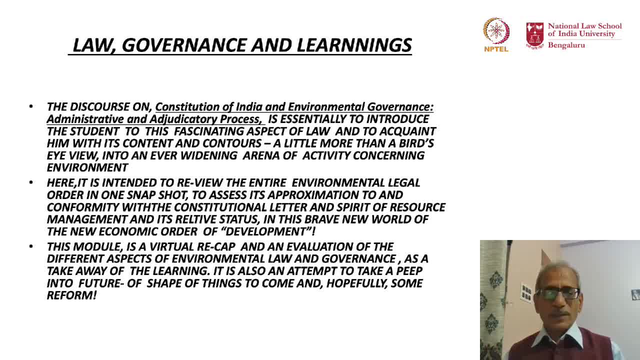 This is a virtual recap and also an evaluation of different aspects of environmental law and governance as a takeaway of this learning, also an attempt to have a gentle peek into the future, future of shape of things to come and hopefully, a few suggestions for reform. 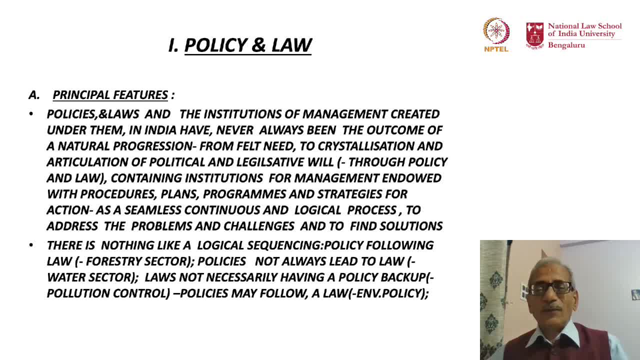 Let us begin with the policy and law as prevalent in India And, if I can just put it this way, I have put it in about 8-10 points as to what are its principle features If you look at the policies and laws and the institution of management created under them. 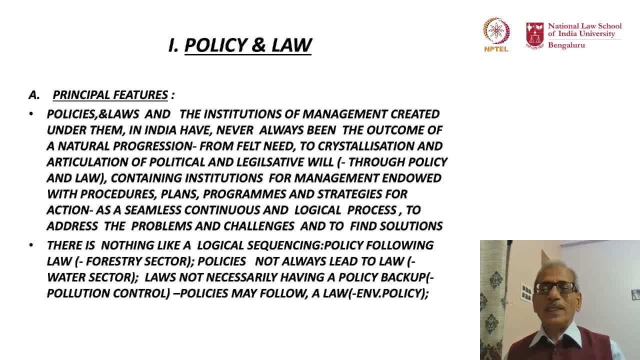 in India. they have never, ever been, at all times, an outcome of a natural progression, a felt need, crystallization and articulation of political and legislative will as reflected through a policy or a law, Having within it institutions for management which is embellished with procedures, plans. 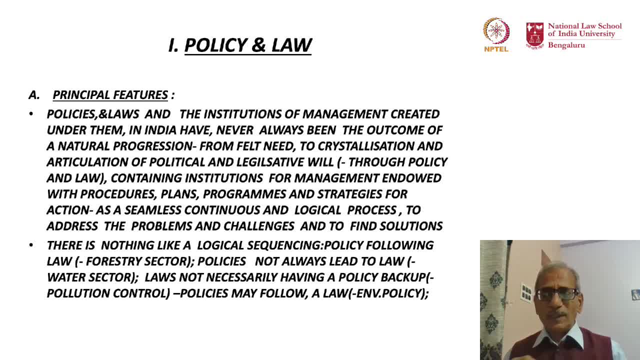 and programs of action as a seamless, continuous and logical process to address the problem and find solutions. but none of this, as you have witnessed so far, has been the feature of Indian policy and law concerning environment. There is nothing like a logical sequencing of this kind of policy, following the law. 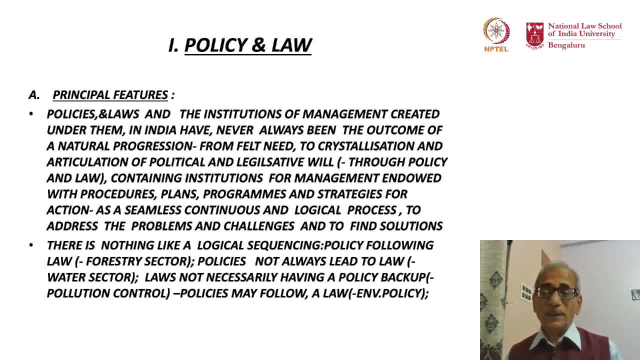 Yes, we have an example in the forestry sector. law came earlier, in 1879, policy followed it in 1894, and policies do not always lead to law. Look at the water sector. Look at the water sector. In 1988 we came up with a draft policy 2002, another policy 2012, another policy where. 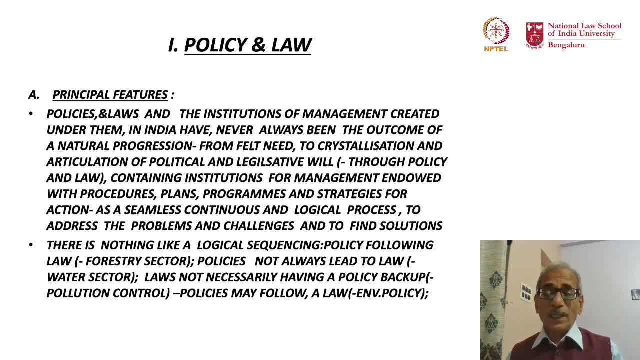 is the law. Laws are not necessarily having a policy backup also, So there can be a law without a policy backup. yeah, Nothing exaggerated here. As you have seen for yourselves: the Water Prevention and Control of Pollution Act and Air Prevention and Control of Pollution Act. 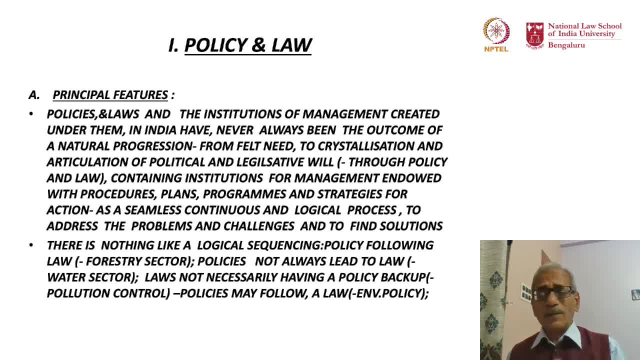 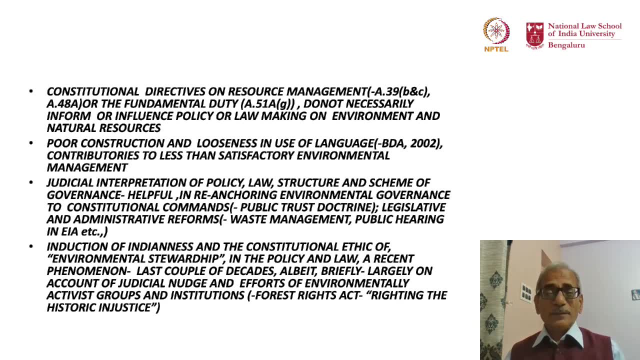 Did not have a policy backup. they just came or it is quite possible that policies may follow laws also. The next feature of the Indian policy and law is supposed to be anchored to a constitutional directive, the directive on resource management. The other feature that you notice in the Indian environmental law in terms of the 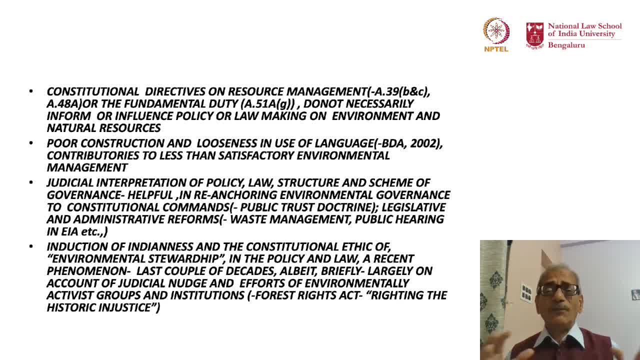 language used and the stuff it is made of. Just to give an example, the Biodiversity Act. Look at the language used, which is quite loose, and the construction of the statue is not that very tight, And because of which, to a large extent, a wonderful law in terms of ideas, but in terms 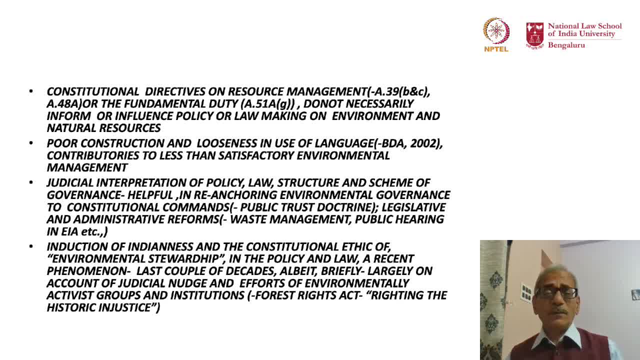 of its construction for the flaws that it has. less than satisfactory environmental governance is the end result. If you turn to the judicial interpretation of policies and laws, you see a silver lining here, At least to the initial stages. very helpful in order to cover for many of the flaws warts. 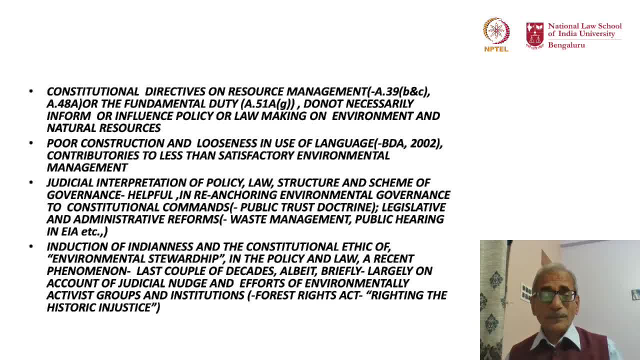 and weaknesses in the construction or making of it or even working. and they helped in re-anchoring environmental governance to constitutional commands, Remember the public trust doctrine and even bring in legislative and administrative reforms on waste management, Even public hearing in environmental tax assessment, as we have seen in the earlier modules. 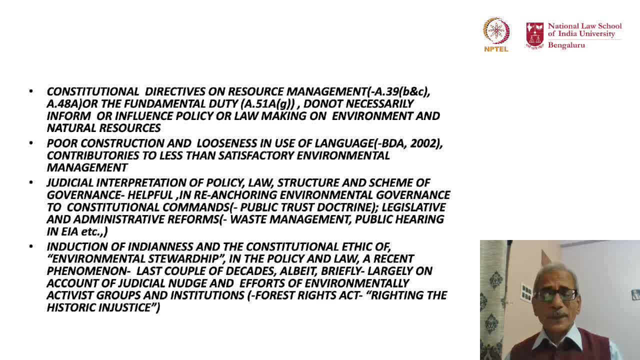 If you closely examine the law as we go deeper, the induction of Indianness and the constitutional ethic of environmental stewardship in the policy and law is more of a fairly recent phenomenon, That too of a last couple of decades, And that is also unaccountable to a large extent on judicial nudge that I and you as 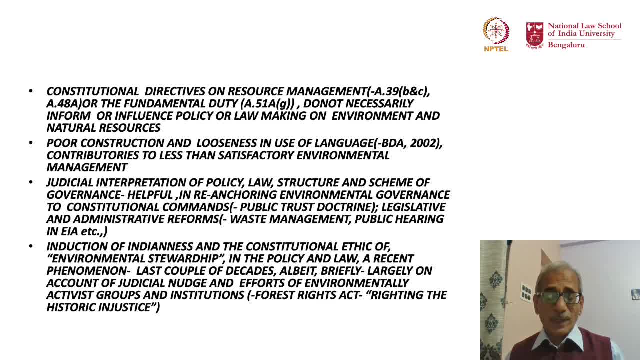 the stewards of the environment is something that the court had to convey time and again, And also, of course, the activist efforts at institutions which actually made people closer to environment and environment, And that is also unaccountable to a large extent on judicial nudge that I and you, as 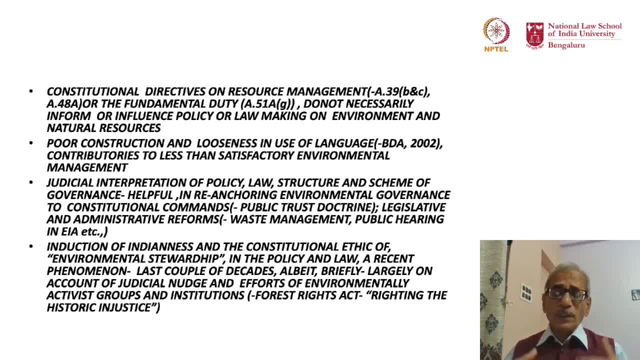 the stewards of the environment and environmental governance And also derive their rights from the kind of laws that environmental laws were made of: The Forest Rights Act, as you have seen made in the year 2006,. declared that this is the law to correct the historic injustice of non-recognition and derail of rights of the forest dwelling. 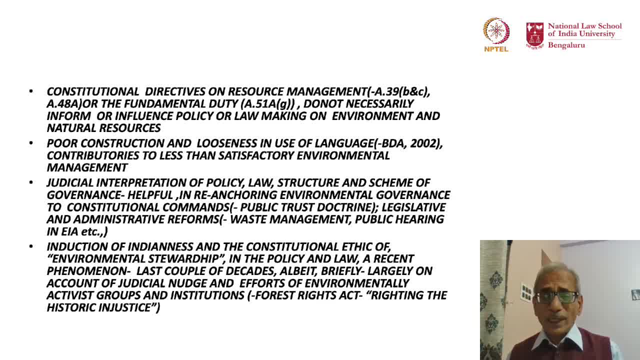 tribal and other species communities. So that way you do have a judicial trigger to lead to the people's engagement, people's involvement, communitarian ownership, communitarian entitlement and partnership in managing environment. Let us just turn a little specific. 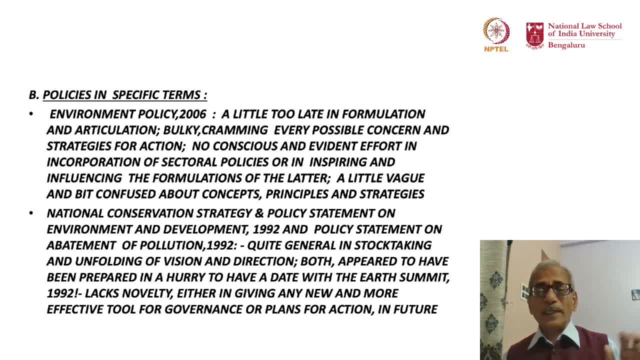 In terms of policies, pick the example of the Environmental Policy Document of 2006.. As you know that there was already a lot of law concerning environment, the Framework Law of Environment Protection Act was made two decades earlier, as early as 1986.. 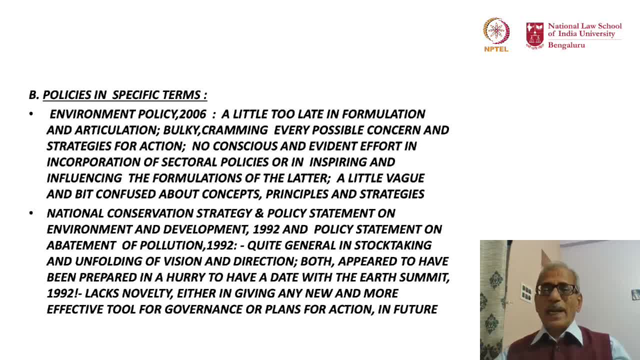 No policy backup and no policy comes makes a very grand entry, although it is a little too late in its formulation and articulation. A bulky document of 60 pages cramming every possible concern and strategies for action, But it is more of a peroration and if you closely examine the document, 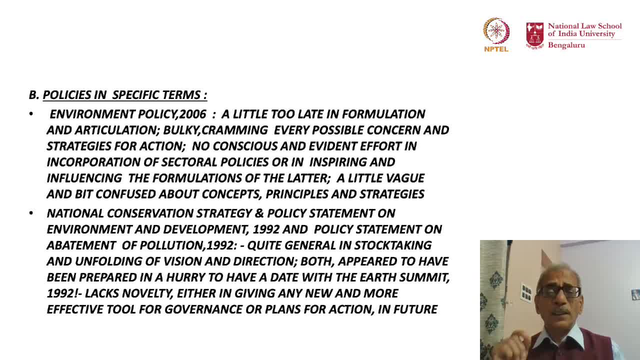 there does not seem to exist a very clear, concerted, conscious and evident effort in consolidation and incorporation of various sectoral policies, or even in inspiring and influencing the formulation of the sectoral policies in different sectors of environmental governance, Even with regard to concepts, principles and 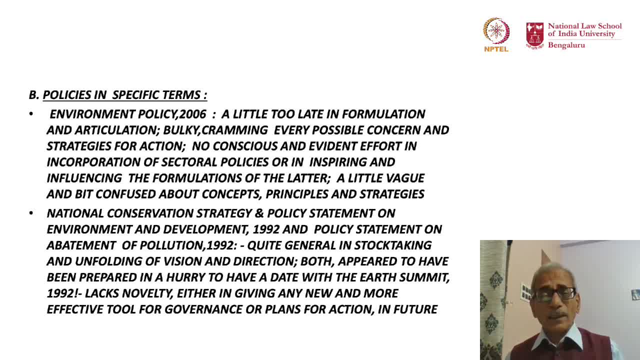 strategies. you find the document a bit vague and confused. The other document- an important policy document, if you want to call it, although the title is a little interesting, if not vague- National Conservation Strategy and Policy Statement on Environment, Environment and Development, made in 1992, and the Policy Statement on Abatement of Pollution. 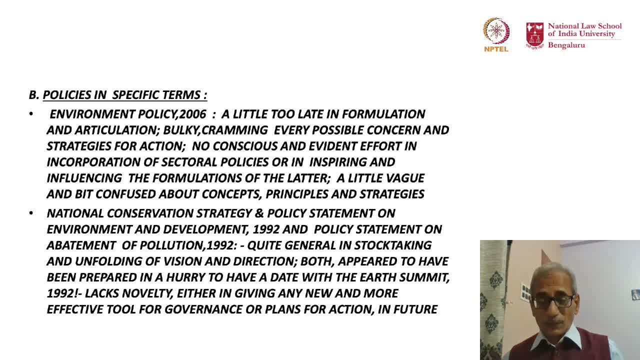 You have such a huge document. looks like title wise, But if you just look to the content, part of it- actually it is of a few pages and it is quite general in terms of taking stock and even a little sketchy in unfolding of a vision and a direction. 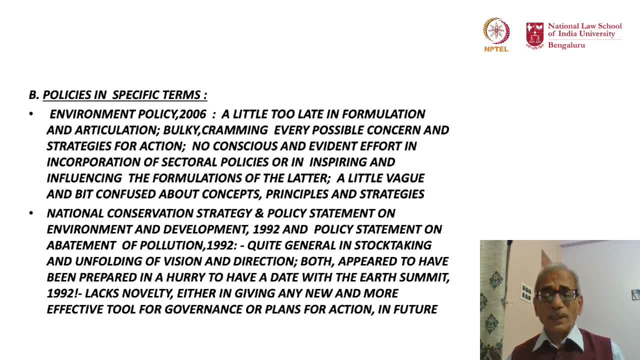 And one would not be wrong in drawing a conclusion that these appear to have been prepared in a hurry to meet the date, Which is the date, The date of the Earth Summit, if you recall the 1992 Global Environmental Summit on Environment and Development, And so we were to go there. 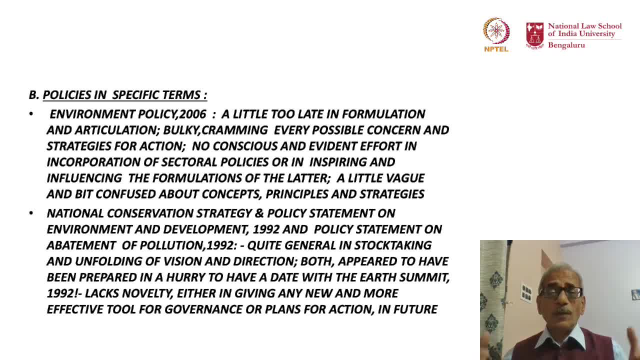 participate in it and we had to show to the rest of the world that we are doing something on the policy front. and hastily we prepared a document and, lo behold, you have this conservation strategy and policy on environment and development and a statement on abatement of pollution. 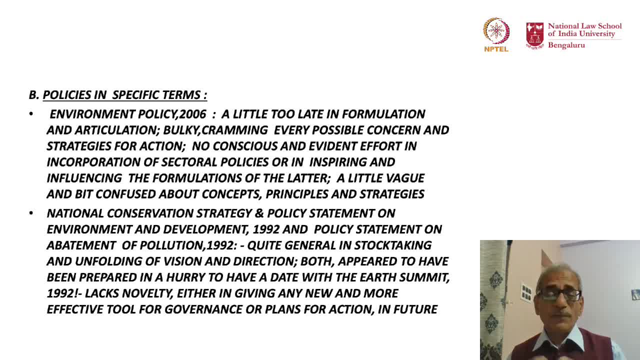 Title grand, eloquent, but content very deficient. There is no nobility either in giving a new thrust or coming up with a novel and effective tool for governance. put together in this document. What you do see is there is more of emphasis on preventive action. 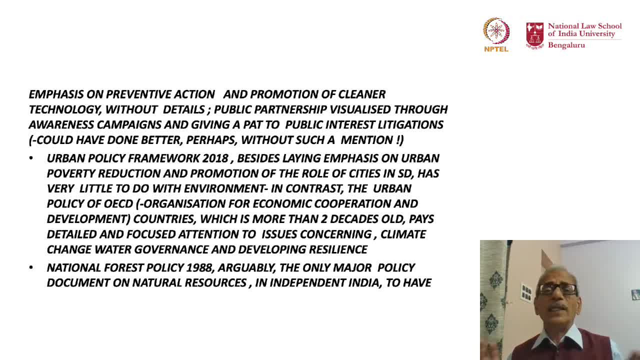 and promotion of clean technology without giving any details there. And there is also a talk about public partnership there in these documents, but it is visualized more as an awareness campaign. I do not know how you forge partnership through awareness campaigns And funnily it is there in this document of giving a path to public interestоб. 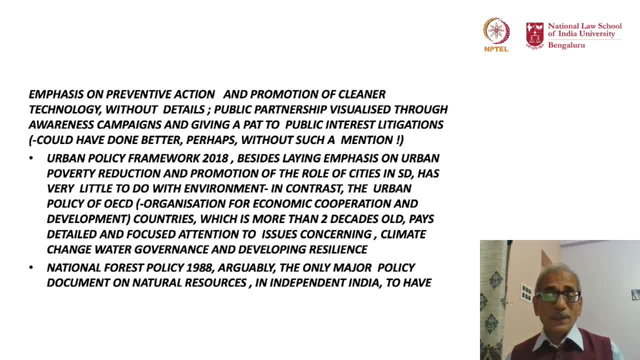 In fact, one is not wrong in feeling that this document, that if at all it were to have been minutely scrutinized in a global summit, they could have better avoided such a kind of a mention, at least this part of it. Then we move to the next policy document, which is fairly, fairly recent, and that is with 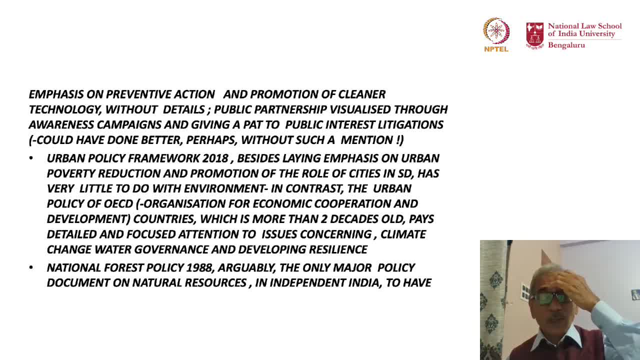 regard to urban policy, It is a framework document of 2018, 2018. yes, did we have a policy frame earlier? Yes, in patches and bits, but not a comprehensive one, and that is what we get now in 2018.. 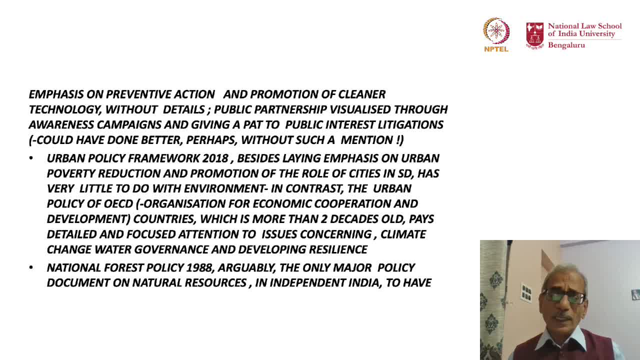 What does it do? It lays emphasis on urban poverty reduction and promotion of the role of cities in sustainable development, And these are the only things that have something to do with it. Let us do a bit of a contrast: How such policies are written, articulated, and how they are put into application. 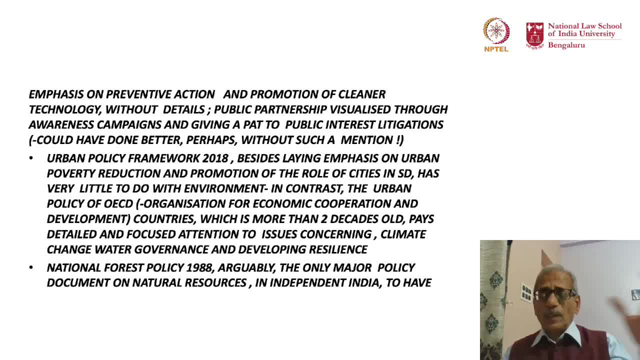 In the Organization for Economic Cooperation and Development, the European group of nations. they have a policy document which is made two decades back And it does not exist. It pays a detailed and focused attention to issues concerning climate change, water governments and developing resilience. 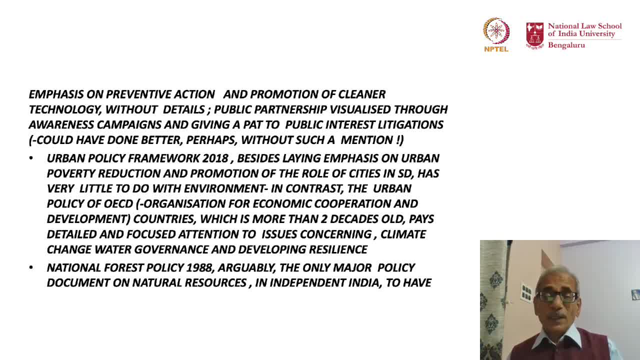 That is what you look for, because urban agglomerate that we have is the real source of huge, huge pollution, waste and all that which is environmentally degrading, And so you should have It had a sizeable section of it, of the policy document getting devoted to environmental conservation. 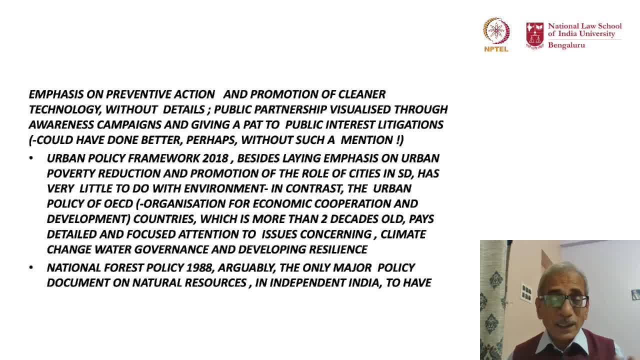 and protection, restoration and recovery- hardly there in this document. Then we get into something which is a kind of a show piece, the National Forest Policy of 1988.. In my reckoning it is perhaps the only major policy document on natural resources as it. 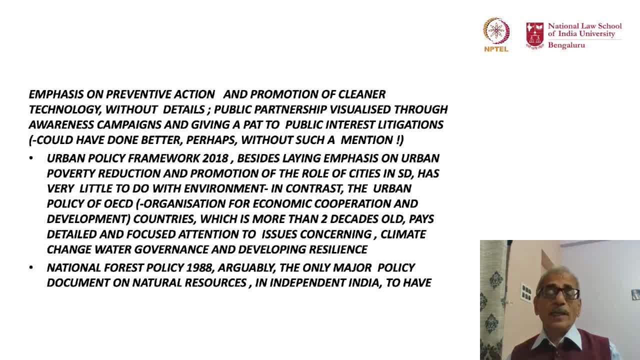 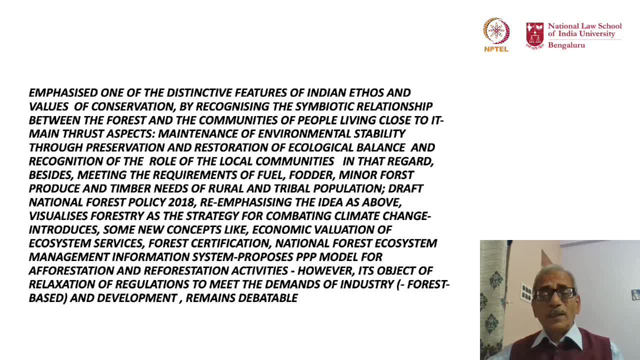 natural resources in India at that point of time, And this is one of those very few policy documents that lays a lot of stress on the distinctive features of Indian ethos and values of conservation. By doing what? By recognizing the symbiotic relationship between the forests and the communities of 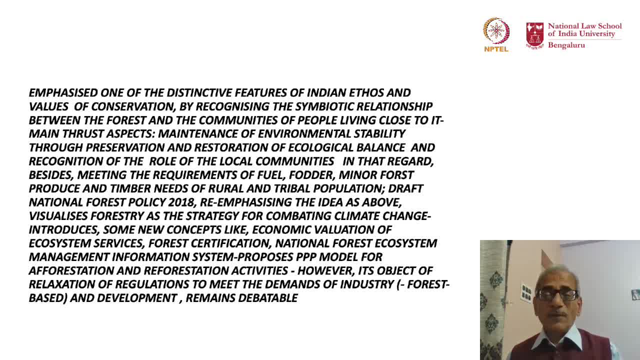 people living close to it. maintenance of environmental stability through preservation and restoration of ecological balance, and recognition of the role of local communities in that regard. In addition to enabling and facilitating the meeting of requirements of fuel, fodder, marine and forest produce and timber needs of rural and tribal population, embellish this document. 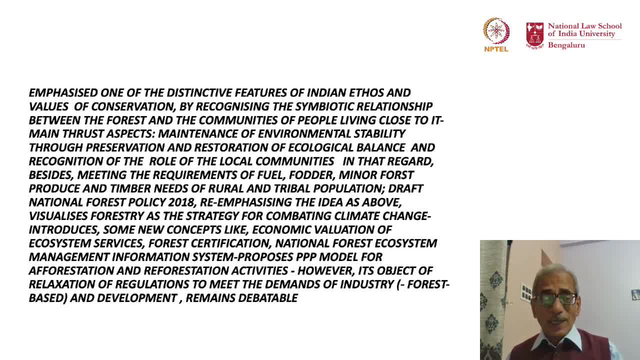 The policy document, by re-emphasizing these aspects which are very basic, which actually bring the connect between the people and the forests, visualizes forestry as a strategy for combating climate change. This comes in the year 1988. And remember, The climate change convention, the framework convention, comes only in the year 1992, four: 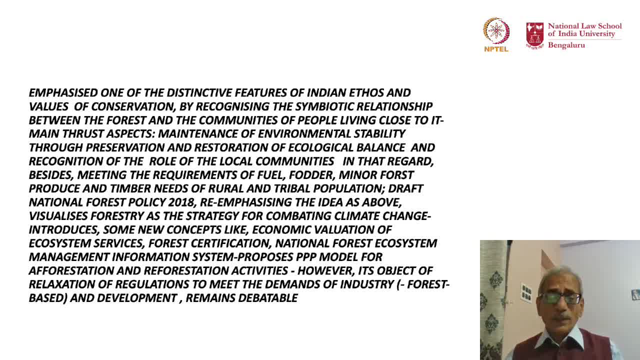 years hence. It introduces some new concepts, as it happened in 2018, the new document, which is 30 years advanced to what was done in 1988, which introduces novelty of strategy for combating climate change. It introduces new concepts. It introduces quite a few new concepts. 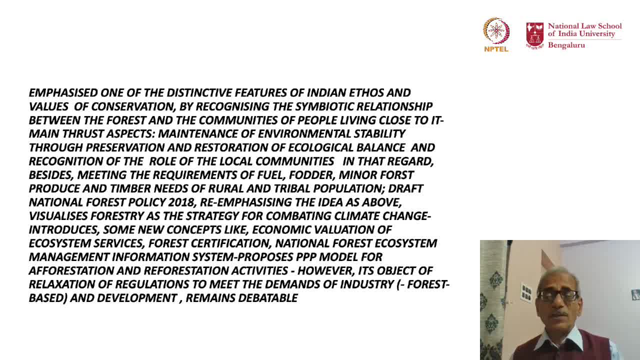 Economic valuation of ecosystem services, forest certification, national forest ecosystem management information system. All these appear to be a fairly advanced approach to forest conservation and management, and it looks like a very professionally evolved document of 2018.. Thank you. It proposes a public-private partnership model for afforestation and re-afforestation. 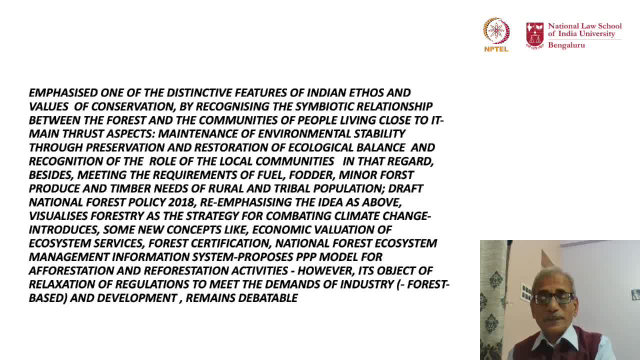 activity. There is a summer note here. It is object of relaxation of regulations to meet the demands of development and especially those industries which are forest based. It is a bit debatable, Okay, It is a bit debatable for the simple reason that you have a different vision of the forest. 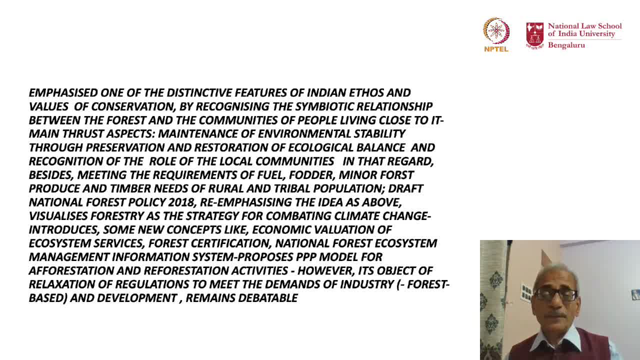 and we had discussed in great detail what are forests for. While the first part- all that we have discussed so far as has been reflected in the 2018 document- appear pretty good, the latter part gives room for a little doubt as to why for this. 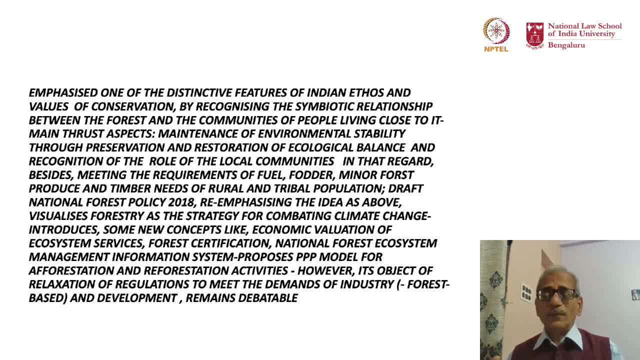 policy has been made, Is it to promote certain kinds of development which will actually have an adverse impact on the forest coverage, the quality and intrinsic value and worth of the forest resources? That requires A little bit more debate. luckily it has not become a deep policy document. it is more. 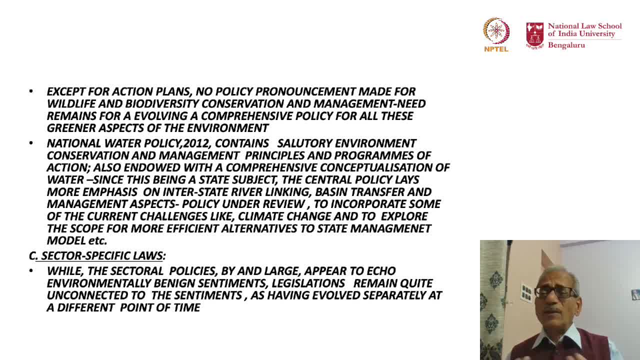 of a draft. Other than that, there are more action plans available. There is no policy announcement made for wildlife and biodiversity conservation and their management, although we have laws on that, and the need remains for evolving a comprehensive policy that would cover all these greener aspects of environment. 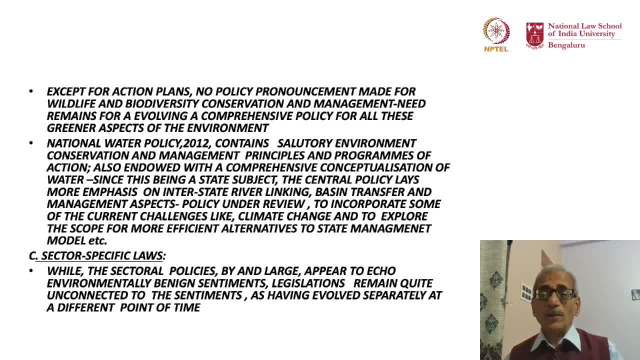 Still the agenda Is not accommodated. Then you turn to the other natural resource of water, with all those tentative attempts of 1988. and then some kind of a formulation, a centre making itself brave to foray into the state subject and come up with a model policy document in 2002 gets revised in the 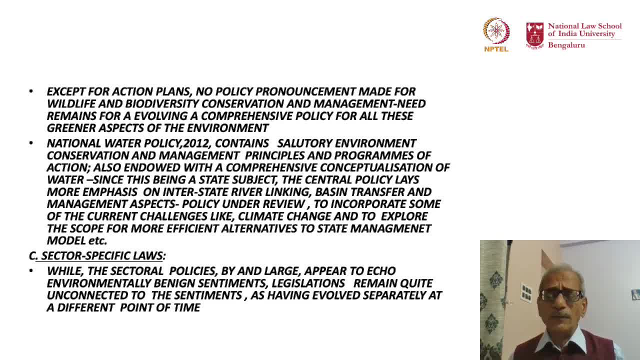 year 2012.. And definitely contains very important information. So that is the agenda. Thank you very much. Thank you, Sir. Thank you very much, Mahesh, Thank you very much. We will end with a very intensive discussion on conservation of water resources. 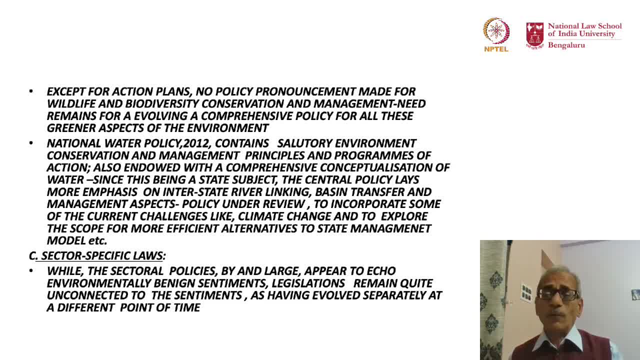 And I will leave you with a very impressive components of environmental conservation and management, principles and even programs of action. In fact, it is also endowed with a very comprehensive conceptualization of water. How should? how to visualize water and not to really think in segments or compartments? 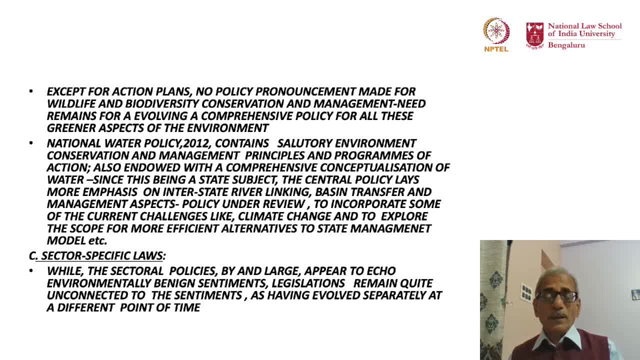 but as one single, continuous whole of an ecosystem. Okay, Okay, Thank you very much. Thank you. The central policy is supposed to be a frame, a guidance document for the states to follow. But to bring in that central element, this policy emphasizes more on interstate river linking, basin transfers and management aspects. 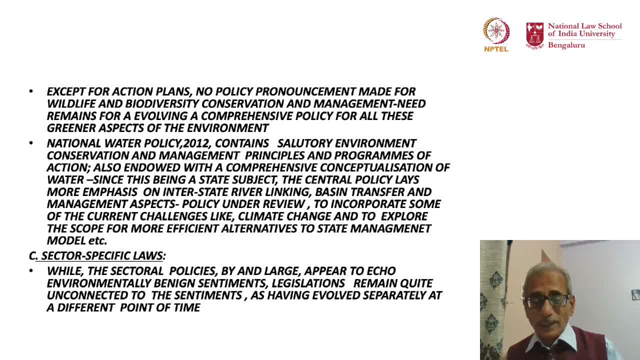 This policy of 2012,. right now, in this year 2020, is under review And the idea is to incorporate some of the new current emerging challenges, like climate change, and to explore scope for more efficient alternatives to state management model, etc. So water policy is still a house under construction. 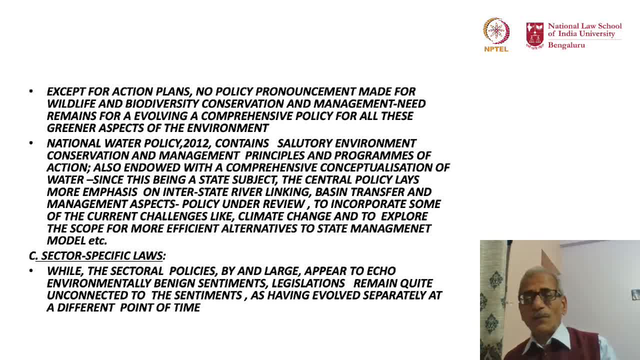 If that is the overview of the policy documents, that we have A quick Look at the sector specific laws, At least we have to give it to the policy documents- by and large Echo that sentiment Of Activities and actions and visions for more an environmentally benign set of activities. 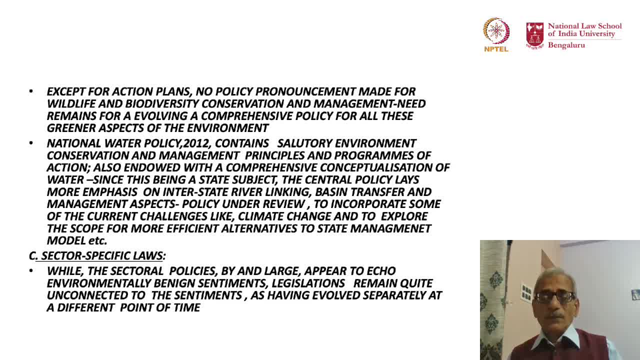 But unconnected to these sentiments. We have laws made for the simple reason that Laws are made at different points of time. So, in terms of accommodation or absorption of policy sentiments is not something that you always look for when you look at a law. 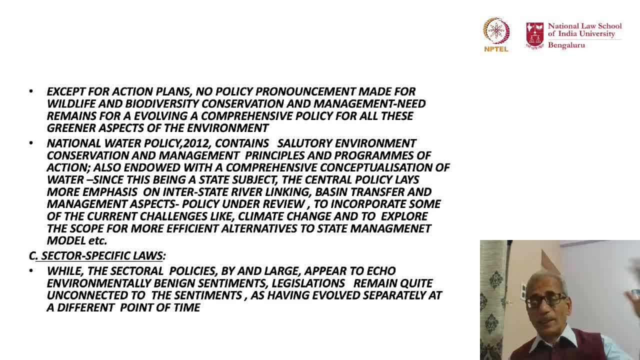 As I have explained earlier in fairly great detail in the specific modules on these, that there is a clear disconnect between policies and laws and many a time you start wondering as to the need for that kind of a formulation. But there is a clear disconnect between policies and laws and many a time you start wondering as to the need for that kind of a formulation. 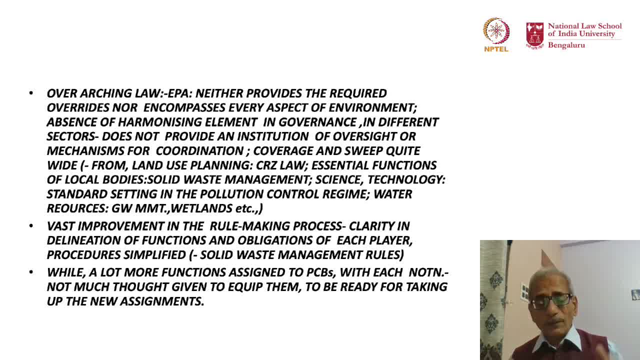 Is it just to fulfill a formality Or is it something to really do very concrete as being really serious about and have a focused attention in having better environmental governments? Look at the overarching law, The environment protection act. What are you looking for? 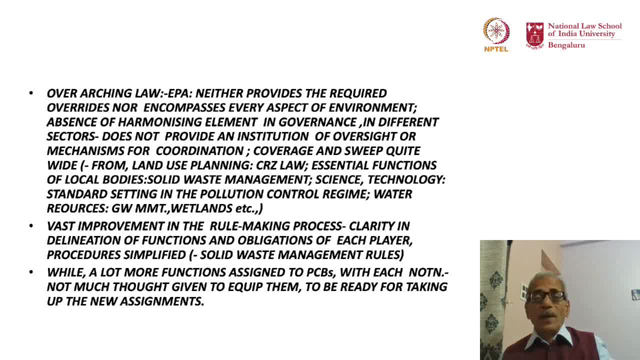 What are your expectations? Something which is all encompassing, But we know that, as we have examined it in detail, It provides neither the required overrides nor encompasses every aspect of environment. I do not think I need to give details. please look to those aspects of the module which 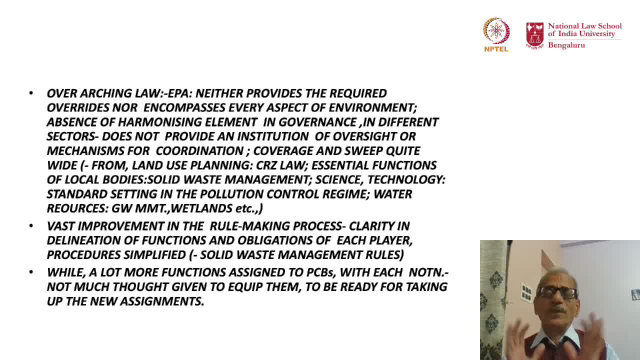 elaborates on this, And there is a clear absence of harmonizing any harmonizing element in governments in different sectors, of knitting them together, meshing their functions, complementing each other's activities into one homogeneous whole. It does not provide an institution of oversight or mechanism for coordination. 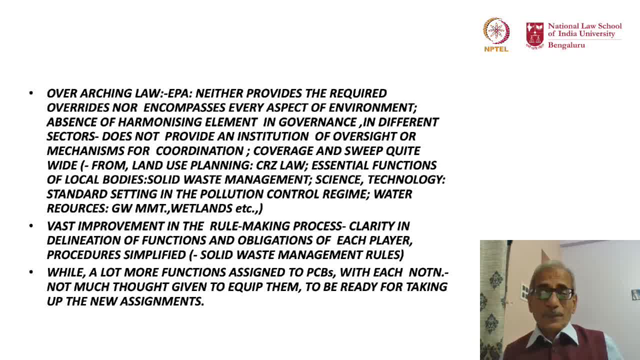 While the coverage and sweep of this body of law, especially the rules, regulations and notifications made under it, are pretty impressive and very wide- Look at that from land use planning under the CRZ law, or essential functions of local body like solid waste management- of incorporating the science and technology aspects, which is 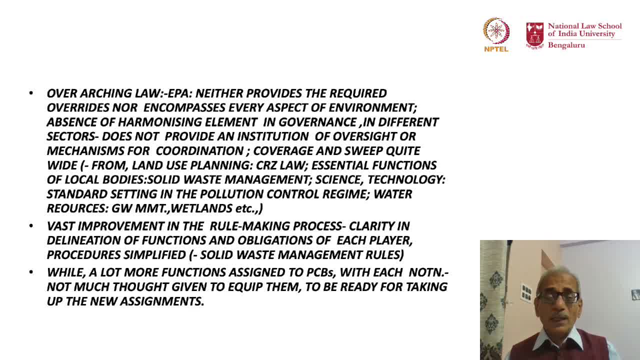 actually the primary realm of the science and technology ministry, like setting of standards in pollution control regime, or even making a foray into water resource management By coming up with rules and regulations with regard to ground water management and guidelines and rules with regard to wetlands conservation, protection and management. the sweep is very 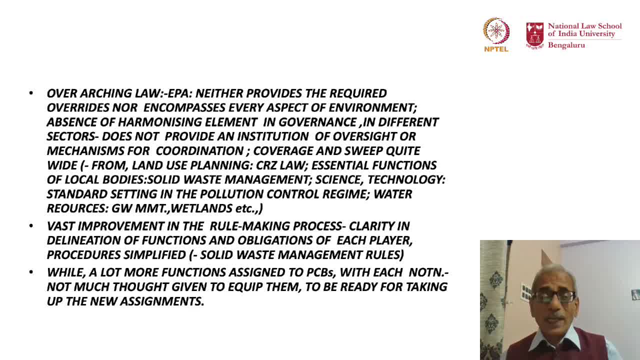 wide, huge and ever expanding, But one thing that you can really deserve, from those early days of law making, from 1986 to maybe till around 2010 or so. So this is what I am talking about. So this is what I am talking about. 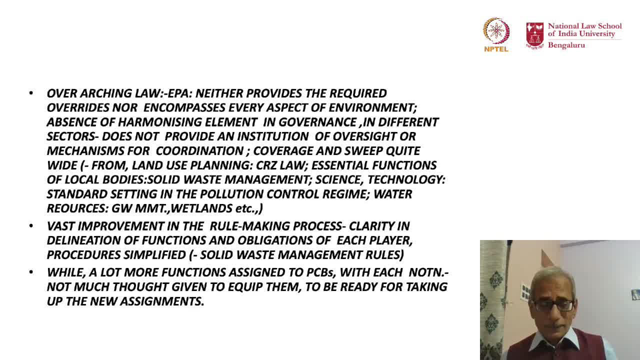 So this is what I am talking about. There is a clear leap frogging, a vast improvement in the rule making process. At least you can see a greater degree of clarity in identification of the actors, their role, responsibilities, functions and a clear delineation of each one of these. 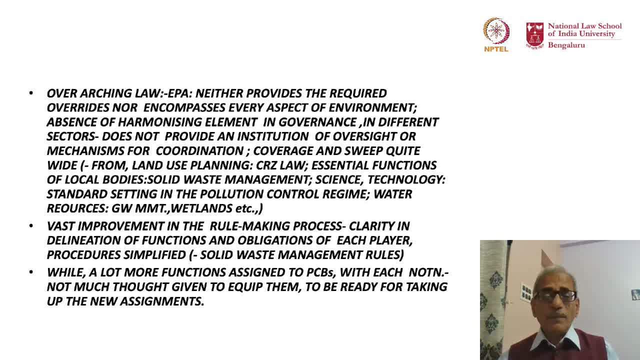 Besides, there is a clear leap frogging. There is a clear leap frogging Besides. there is a clear leap frogging Besides simplification of procedures. One wonderful example that you have is the rules with regard to solid waste management. 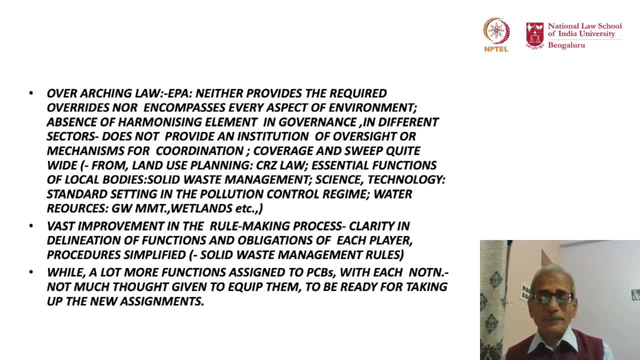 We have discussed that in the earlier module. please refer to that. What you do see is a something unplanned, perhaps unheard, definitely, and something even unprepared as far as the pollution control boards are concerned. a lot more functions are assigned to the pollution control boards with each and every notification. 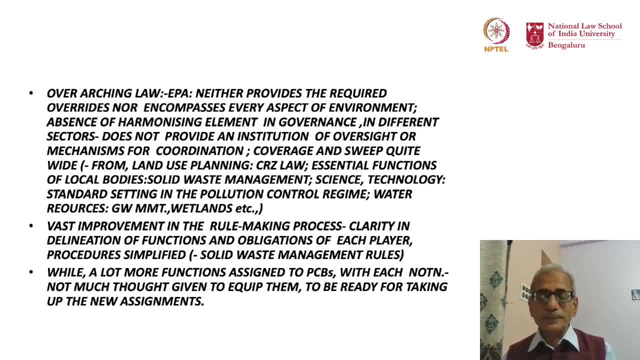 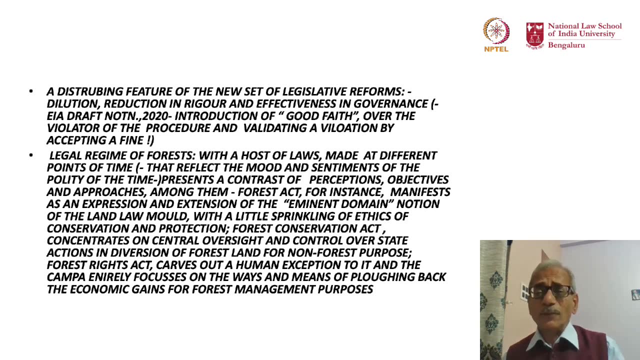 But not much thought is given. How do you equip them? How do you facilitate their functioning? How do you build their capacity When they take up? This is new and ever growing portfolio of assignments and disturbing feature of new set of legislative reforms. also, we have witnessed there is a clear dilution, reduction in rigour. 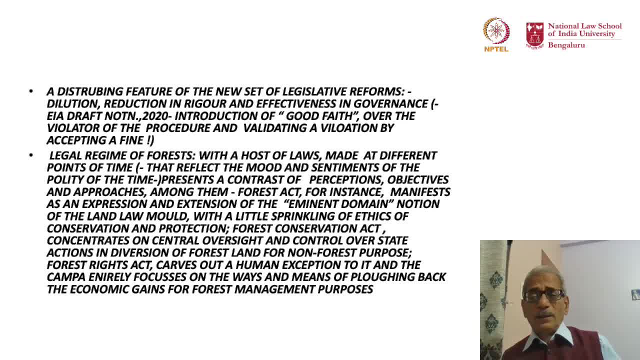 and effectiveness in governance. Look at the notifications with regard to environment impact assessment, and the latest one is something mind blowing: The EIA draft notification of 2020,. you know what it does? It introduces the good faith clause. over whom? Good faith? over the violator of the procedure? and validating a violation by accepting a 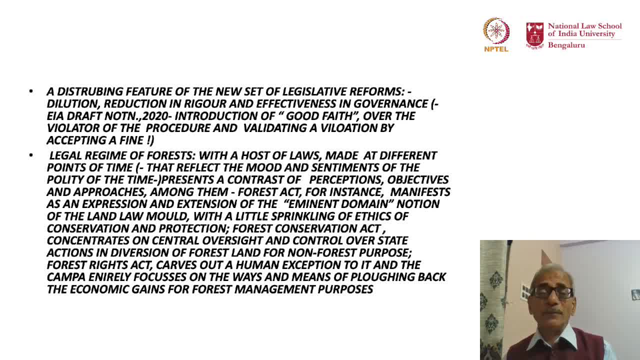 fine. Many a time you start wondering whether such a kind of thing would really do justice to the very idea of environment impact assessment, the rationale behind making such a kind of a law. These are a few worrisome features as they are emerging now. 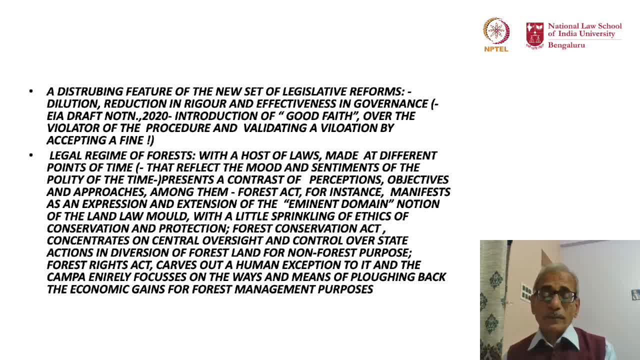 Turn to the legal regimen for us. You have a clutch of laws, and each one of them are made at different points of time, and this is very educative: The laws made at different points of time. The laws made at different points of time. 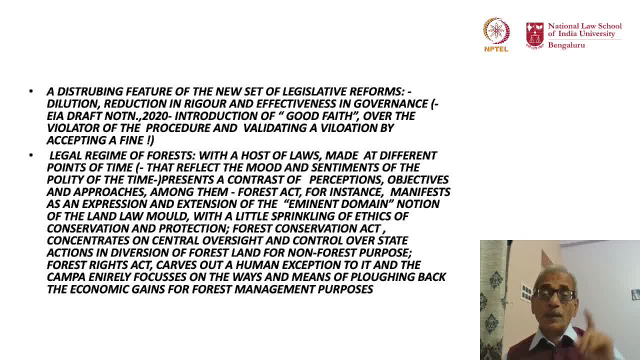 They reflect the mood and sentiments of the polity of the time, right from the time of the British to immediately after independence, a quarter century later, and then fairly recently in this particular decade. they really reflect the trust, the emphasis and the approach of the policy maker, the law maker, the decision maker of the time. 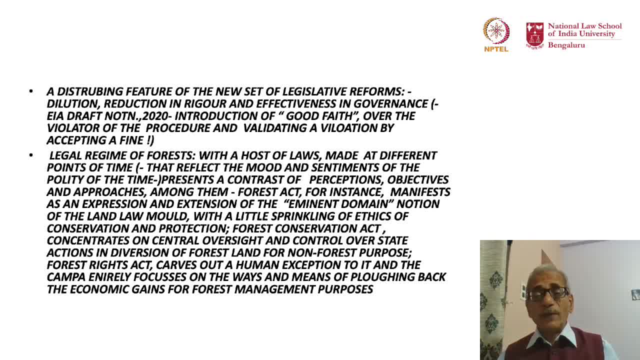 Obviously. as a result, it presents a contrast of perceptions in terms of objectives and approaches. among them, For a fact, for instance, manifest an expression and extension of the eminent domain notion State owns everything, A notion Which it derives from the land law scheme with a little sprinkling of ethics of conservation. 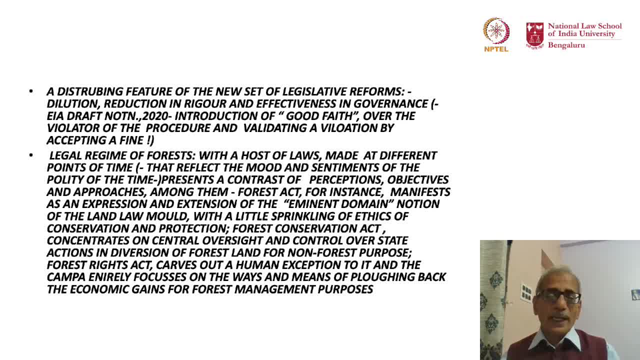 and protection. Turn to Forest Conservation Act. Its focus is on central oversight and control over state actions with regard to diversion of forest land for non-forest purpose. The forest rights of the land. The forest rights of the land. The forest rights of the land. 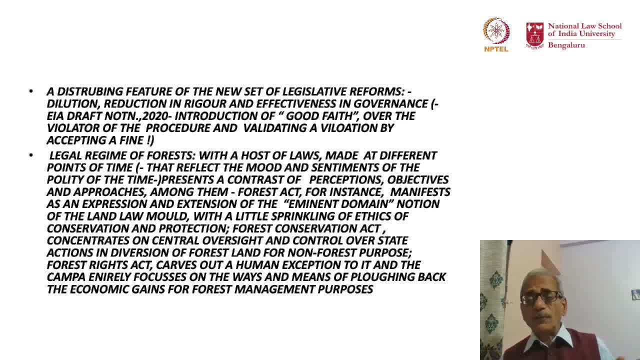 The Forest Rights Act has a different focus altogether. It calls out a human exception to the forest conservation law And the 2015 Kampa Law entirely focus on the ways and means of bringing back and blowing back the economic gains that you derive from the different kinds of applications and techniques. 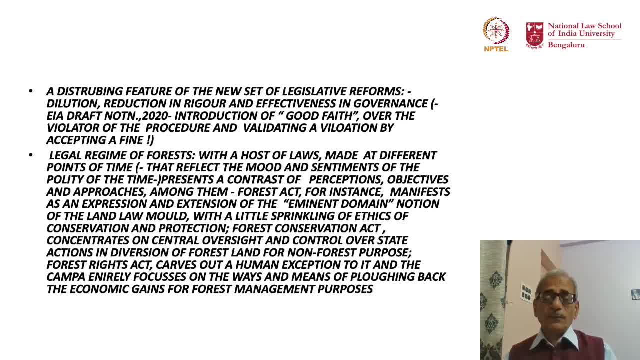 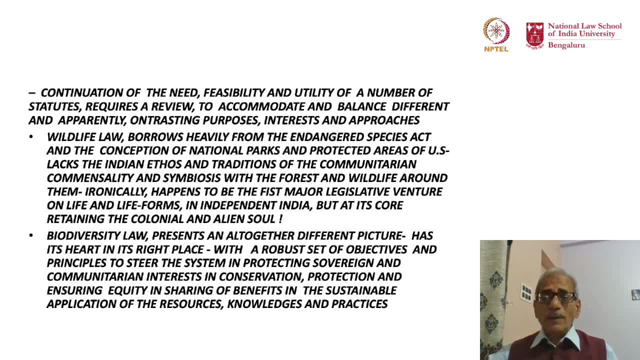 application of forest resources for the purpose of forest management and improving the quality of governments. So different perceptions, different approaches actually populate the entire forest law regime. Continuation of the need, feasibility and utility of a number of statutes of this kind definitely would require a review. 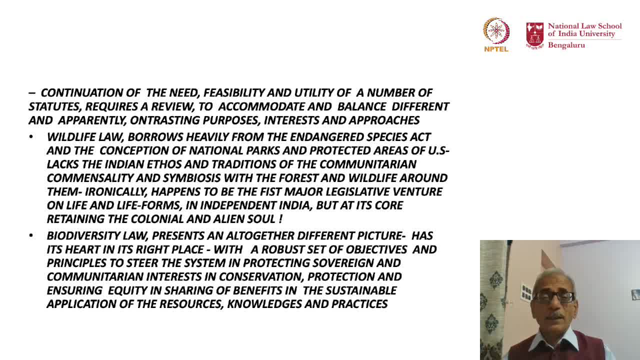 The idea is to accommodate and balance different and apparently even contrasting purposes and interest side approaches. Wildlife law does not do anything better. The wildlife law as we know it it is a clear copy or a borrower of the ideas of the Endangered Species Act. 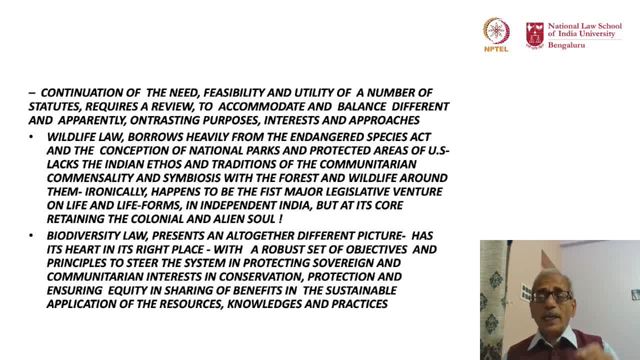 And the conception of national parks and protected areas of United States of America. It lacks the Indian ethos and traditions of the communitarian commensality and symbiosis with the forest and wildlife around them. Ironically, the wildlife law of 1972 and its refurbished law in 2007, the wildlife law 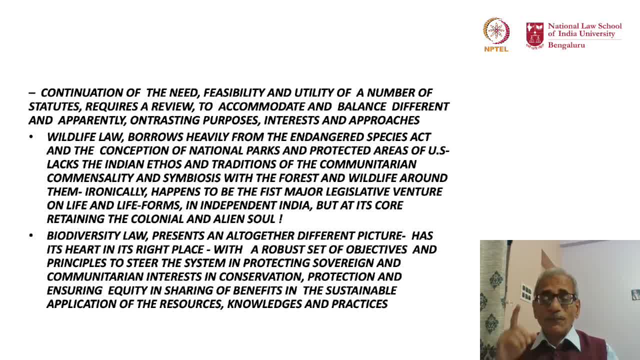 of 2007.. In 2002, it happens to be the first major legislative venture on life and life forms in independent India, But its core- it retains a colonial and Aryan soul. We have already discussed that in that particular module. 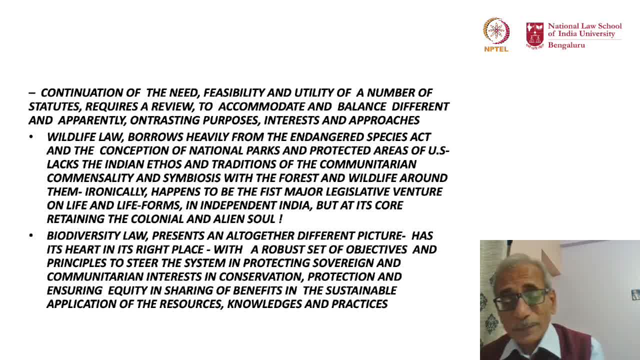 We now turn to the biodiversity law. It is a refreshing departure. It presents an altogether different picture. As you have seen it, it has its heart in its right place, with the robust set of objectives and principles to steer the system in protecting the sovereign and communitarian interests. 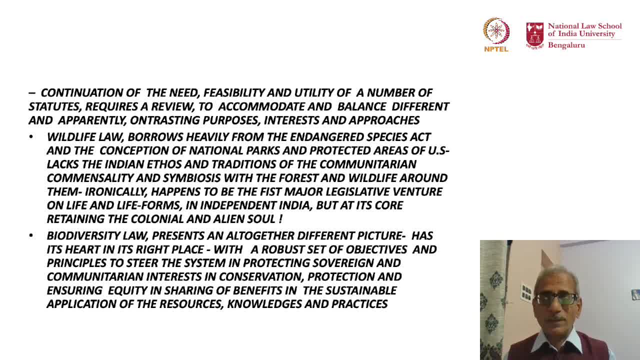 With regard to what? conservation, protection and ensuring equity in the sharing of benefits. okay, benefits with regard to the application of resources and the knowledges, practices, customs and traditions associated with it. No single law does this kind of a thing as the biodiversity law has been able to put. 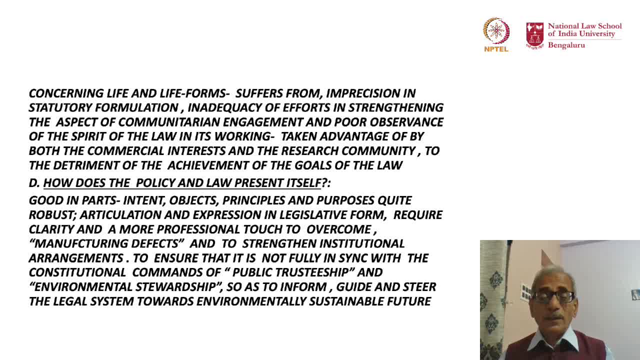 across. Besides this, it actually is a great experiment in deepening democracy, much more than what you find in the constitutional scheme itself. But it is very unfortunate that this is, which is a very great idea. it suffers from imprecision in statutory formulation and inadequacy in terms of the law. 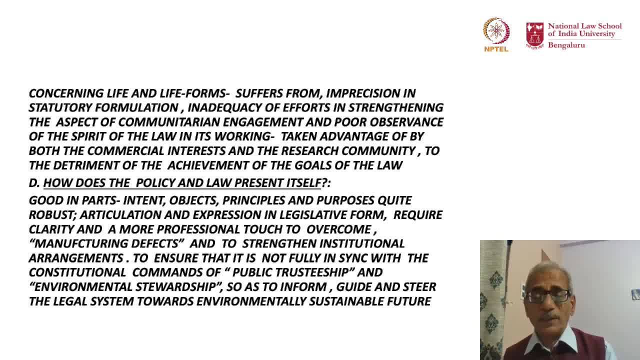 The efforts in strengthening the aspect of communitarian engagement and a poor observance of the spirit of the law in its working by all concerned. and you know the end result. This inadequacy has been taken advantage of by unscrupulous commercial interest, and even 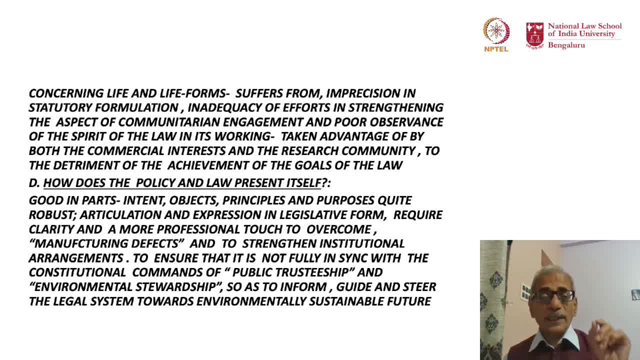 some of the irresponsible research community as well, to the detriment of the achievement of the goals of this project. Thank you. So, overall, how do these policies and laws, wrap up together, present themselves in the Indian firmament? Yes, they are good in parts in terms of objectives. as far as intents are concerned, in evolving